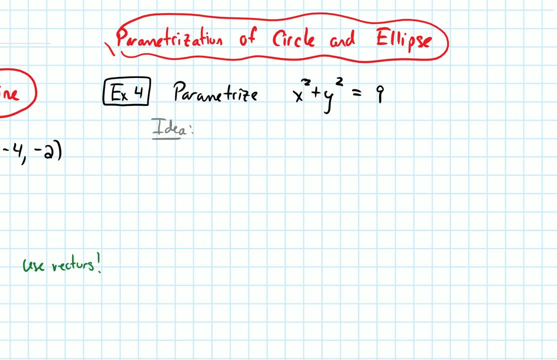 parametrize. this is I know circles. so I know circles sort of remind me of the unit circle, They remind us of the unit circle and the unit circle x sort of corresponds to a cosine and the y-coordinate corresponds to a sine. So also when we see something squared plus something squared and we think of 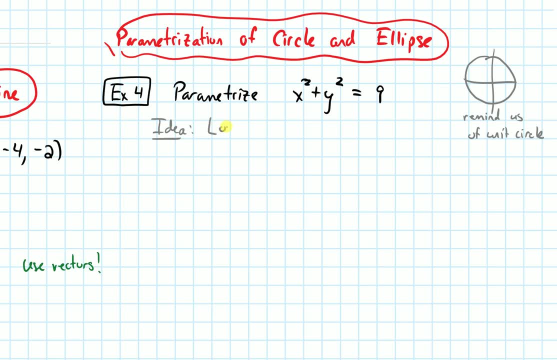 cosines and we think of sines, we think of the fact that this looks like: cosine squared t plus sine squared t equals 1.. So of course it doesn't look exactly like that. So right now I don't have a cosine in here or a sine in here, and I have a 9,, I don't have a 1, but 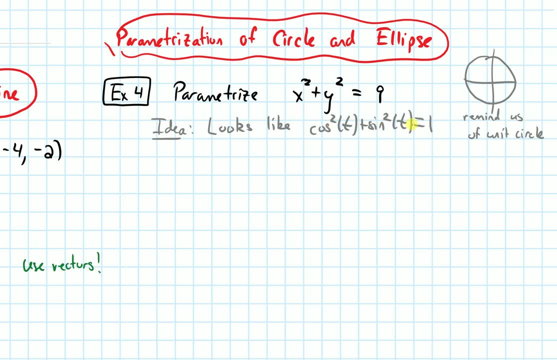 nonetheless, there are two squares being summed and that's equaling some number. Okay, so here's how we can modify that. If we took this equation and multiplied everything by 9 and got 9 cosine squared t plus 9 sine squared t, we would get 9 cosine squared t plus 9 sine squared t. 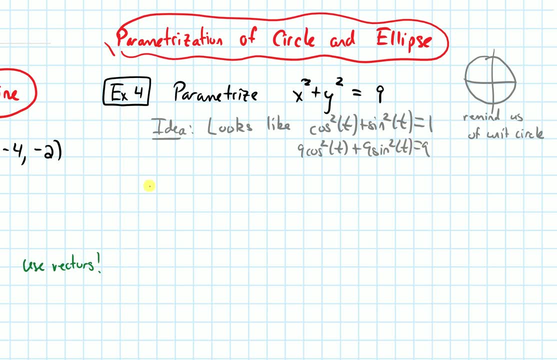 That gives me an idea for what we can let x and y be. So I'm gonna let x be 3 cosine t. That way, when we square it, we're gonna get 9 times cosine squared t. Similarly, let's let y be 3 times sine t. Okay, and when we do this, when we take 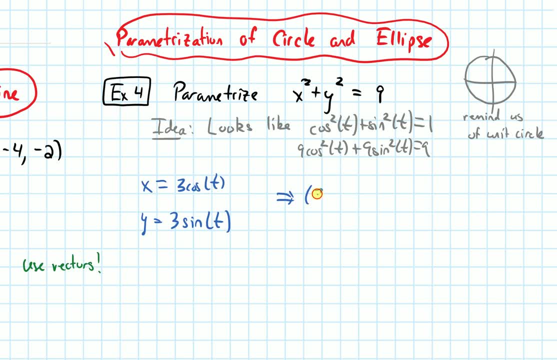 these values and we plug them into this equation, we end up getting 3 cosine of t squared plus 3 sine t squared, and that gives us 9 cosine squared t plus 9 sine squared t, which we know is 9.. So this is gonna work out when we plug it into this. 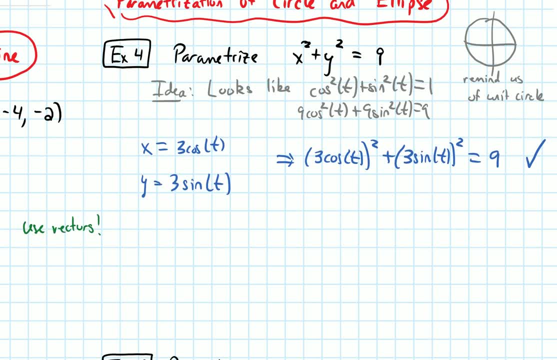 parameterization. Okay. so the one thing I haven't specified at this point is what the domain is and what t, what range of values t takes on. So let's look at a table of values and let's look at those points on a graph to give us a feel for what we want that. 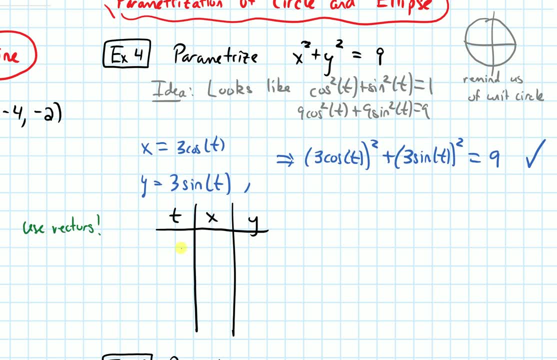 domain to be. So this time when I plug in values for t, I need to plug in nice angles because they have to be plugged into a cosine and a sine function. So let's plug in things like 0 and pi over 4 and pi over 2, and I'll just do those. 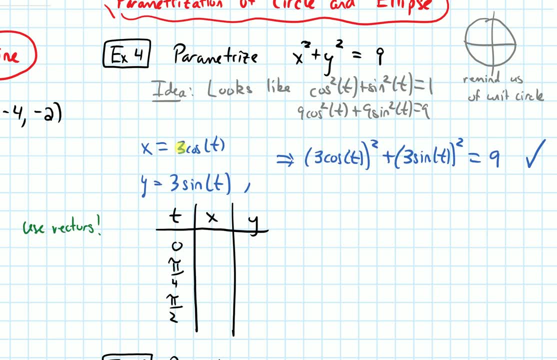 three. So plug in in 0, 3 times cosine of 0 is 3.. If I plug in pi over 4, we'll get 3 times cosine of 0 is 3.. If I plug in pi over 4, we'll get 3 times cosine of 0 is 3.. 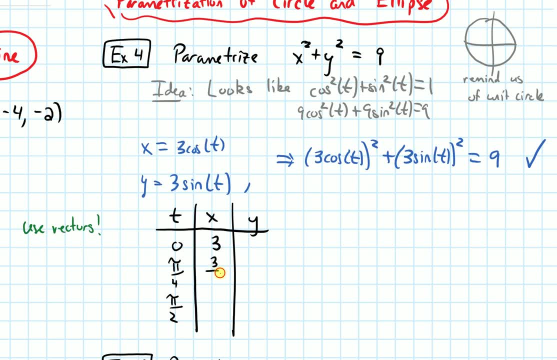 times 1 over root 2, which is 3 over root 2.. Plug in pi over 2. we get 0, because that's what cosine of pi over 2 is. If we do the same thing with the y, we'll get 0 here, because sine of 0 is 0. We'll get 3 over root 2 here. and then, when we plug, 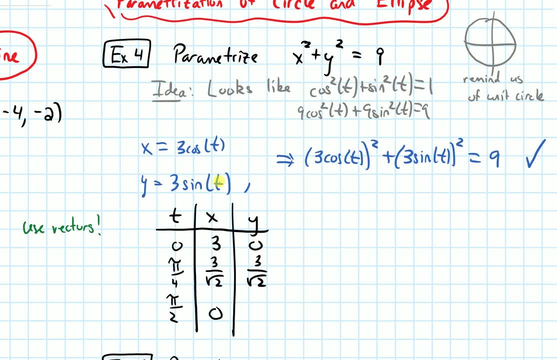 in pi over 2, sine of pi over 2 is 1, and when we multiply that by 3 we get 3.. Okay, so these are a few of the points on this circumference of the circle. So if I draw this circle, so this is where 3 is. on the 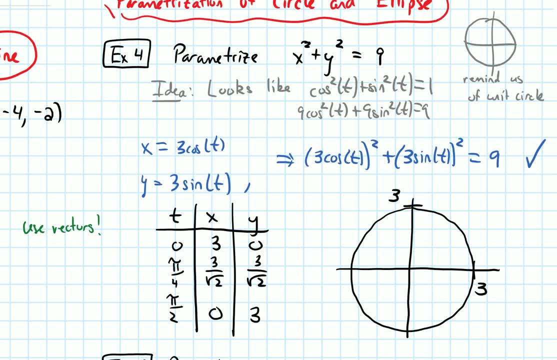 x-axis. this is where 3 is on the y-axis. So when t equals 0, we are here at 3, 0.. When t equals pi over 4, we are at this point where the x and the y coordinates are the same, So t equals pi over 4. and then when t is pi over 2, we are at this. 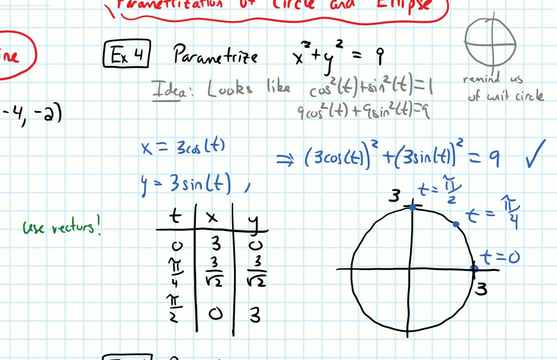 point at the top where the x is 0 and the y coordinate is 3.. Okay, so now let's think about the domain and what we want t to go from. So if I just need to describe going around this circle one time, then I could just say that t is in between zero to 2 pi, and that will 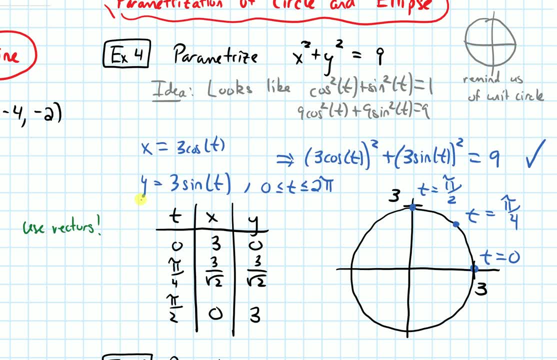 describe going around the circle one full time. So this would be my parameterization right here. I forgot to draw a direction arrows, So my direction arrows are pointing this way and this way and then I keep going around in that direction. So this parameterization gave me this counterclockwise. 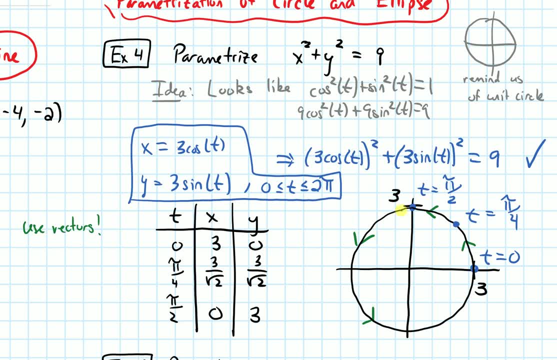 parameterization of this circle. So it's a good warm-up exercise to think about. well, what if I had wanted it to go in the opposite direction? How would I have needed to change this parameterization? Or what if I wanted it to go around the unit circle more than one time? How? 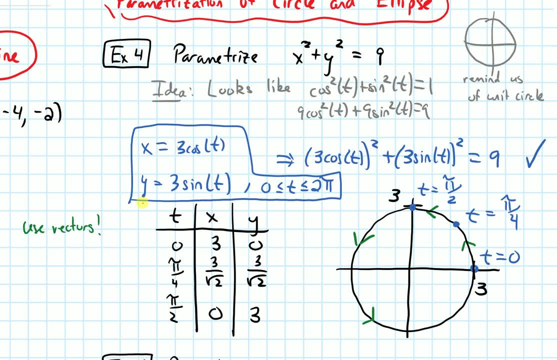 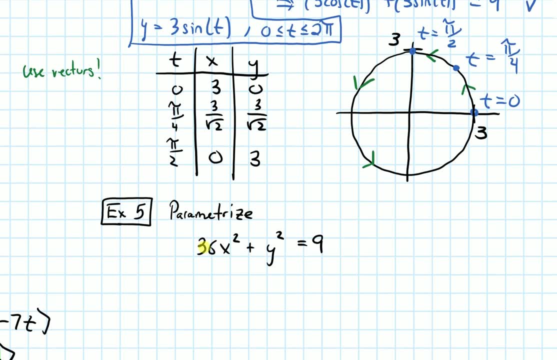 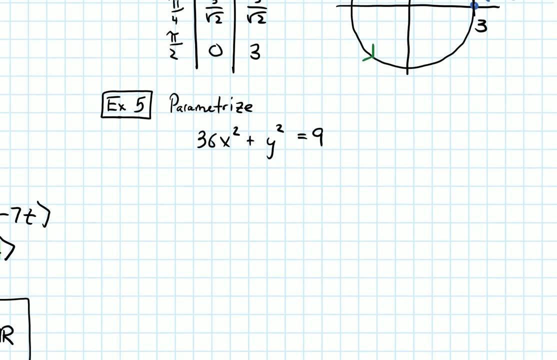 would I have accomplished that with my parameterization, And we'll answer some of these questions in the homework. All right, so let's do another example now. Now let's parameterize: 36x squared plus y squared equals a 9. So this isn't a circle. 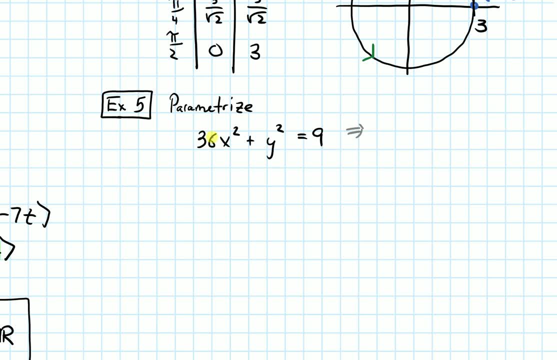 So we might recognize that this is the equation of an ellipse. The equation of an ellipse in general looks like x squared over x squared square plus y squared, So we might recognize that this is the equation of an ellipse. So we might recognize that this is the equation of an ellipse. So we might recognize that this is the. 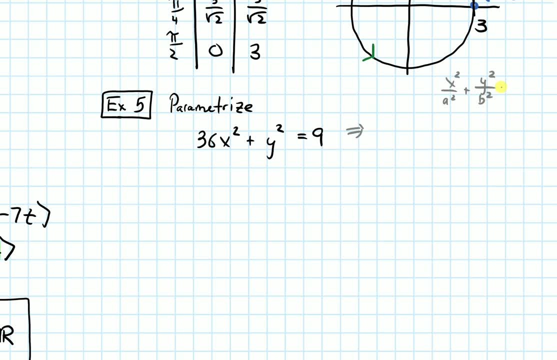 a squared plus y squared over b squared equals 1.. So an ellipse in general has this form And to put it in that form I need to divide by the 9. And that gives us 4x squared plus y squared over 9 equals 1.. And it still doesn't quite have that form because x squared is supposed. 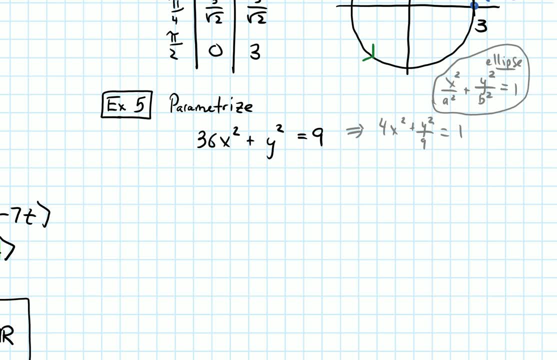 to be divided by a number. But to put it in that form, I just have to rewrite 4x squared as x squared being divided by 1. fourth, And now this has the form for the equation of an ellipse. So how do we handle an ellipse? Because we did circles, but what do we do for an ellipse? 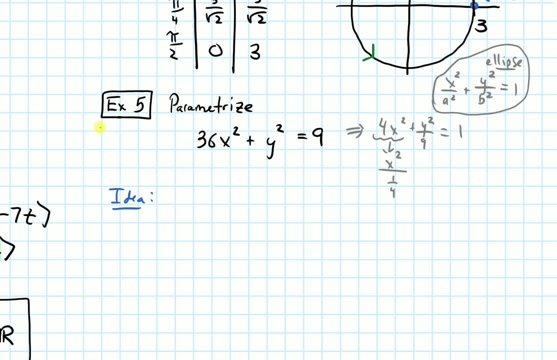 So my idea here is going to be to sort of mirror what we did above, And it would be really nice if this 36x squared, if we let that 36, x squared be equal to 9 times cosine squared t, And then if we let the y squared. so, if we let the y squared, let's put this in a different color. 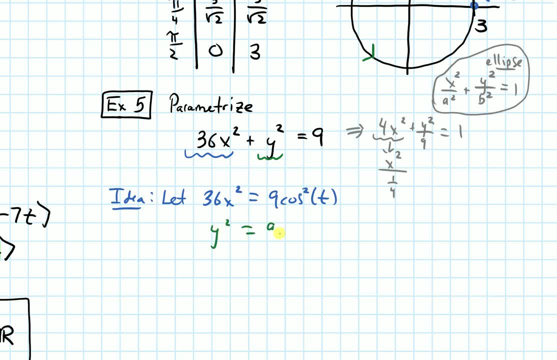 actually, If we let the y squared be 9 times sine squared t, because we already know that 9 times cosine squared of t plus 9 times sine squared of t equals 9.. Okay, So in this first equation, if we isolate, we get 9 times sine squared of t plus 9 times sine squared of t. 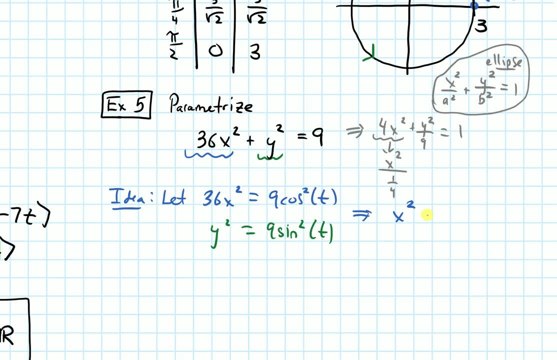 So if we isolate for x squared dividing by 36, we'll get x squared equals 1 fourth- Oh, let's write that four a little bit better: 1 fourth cosine squared t. And now we could square root both of these equations. 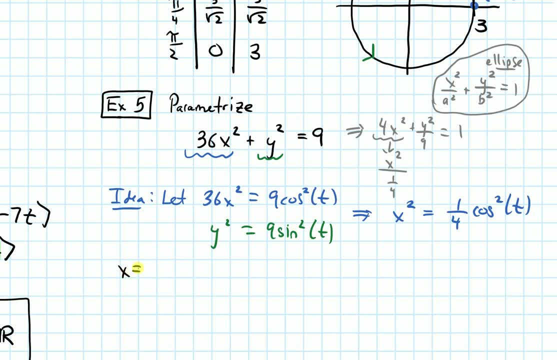 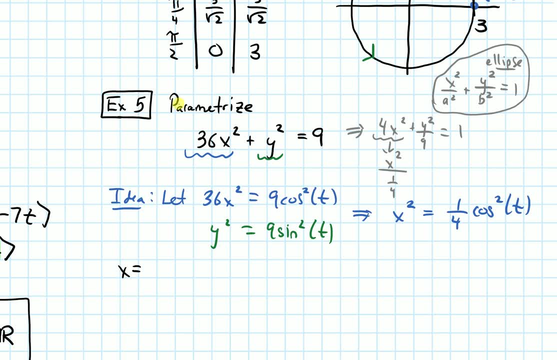 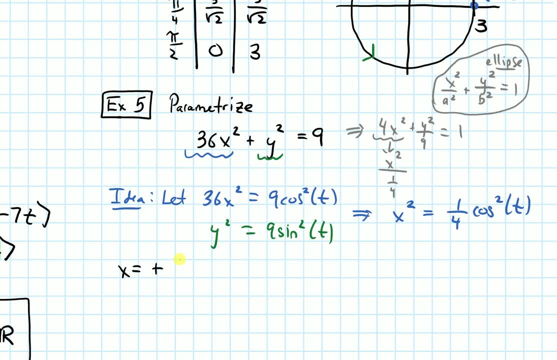 If we chose the positive version, the positive root, 1 half cosine of t, we'll get one parameterization. If we had chosen the negative root, we'll get a different parameterization, but that's okay. So I'm just going to stick to the positive version. Same thing for the y When I square. 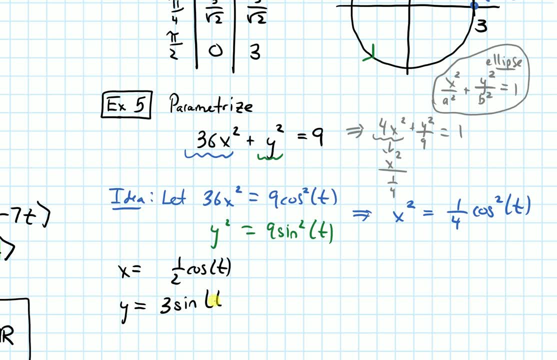 root y squared, we'll get 3 sine t And again, I'm going to let t be between 0 and 2 pi because that's going to account for going all the way around this ellipse In this case just one time. But note we could also choose negative 1 half cosine t if we had wanted to, and negative 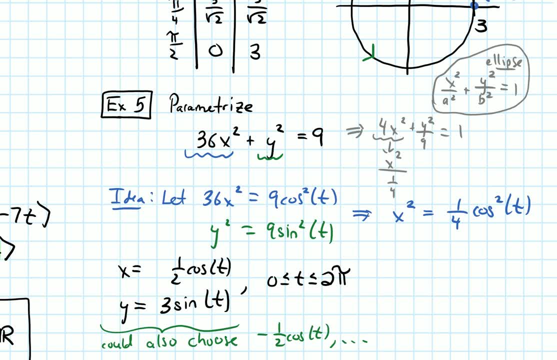 3 sine t. It just gives us a different parameterization, Subtitles by the Amaraorg community, Which might correspond to things like a different direction or a different speed around the curve. Okay, So if we needed to graph this ellipse, if we don't remember things like: 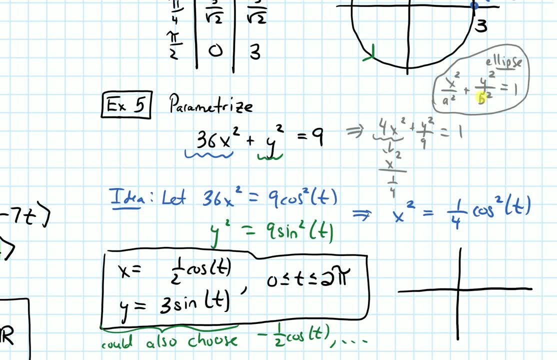 the major axis and the minor axis of an ellipse, based off of what a and b are. we can use this parameterized form to quickly get you know how far across the x direction it goes and how far across the y direction it goes. 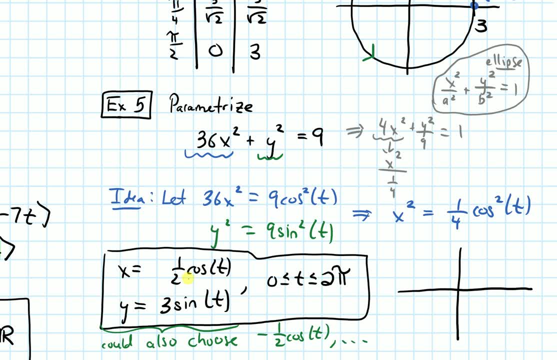 So cosine in general just on its own is always between negative 1 and positive 1.. If we multiply it by 1 half that's always going to be between negative 1 half and positive 1 half. So in the x direction my ellipse will go all the way to negative 1 half in this direction, to the left and to positive 1 half in the right direction. 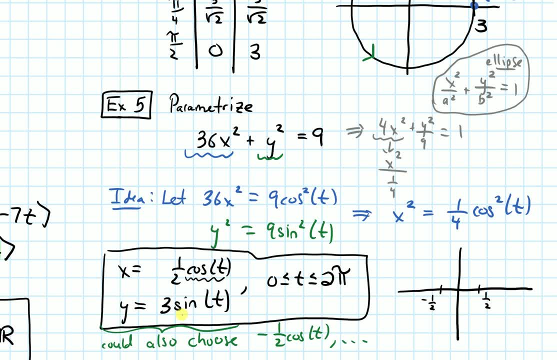 And then sine is also between negative 1 and positive 1.. So multiplying that by 3, it'll mean that y is in between negative, 3 and negative 1.. Let's just write this down: y is going to be between 3 and negative 3, and x is going to be between negative 1 half and positive 1 half. 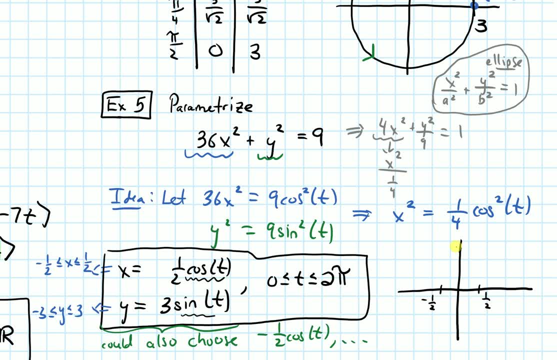 So now we can see that it stretches a whole lot more vertically than this one does horizontally. So my ellipse would have looked something like going down and then back through that point at 1 half and then up. So it's this narrow ellipse here. 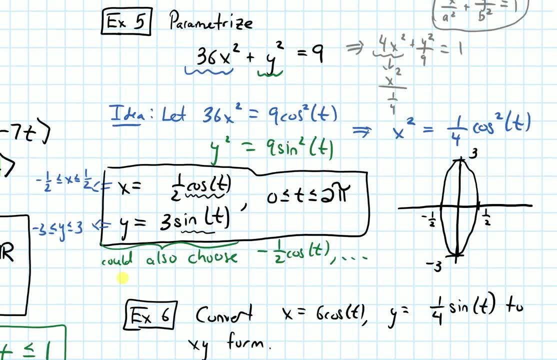 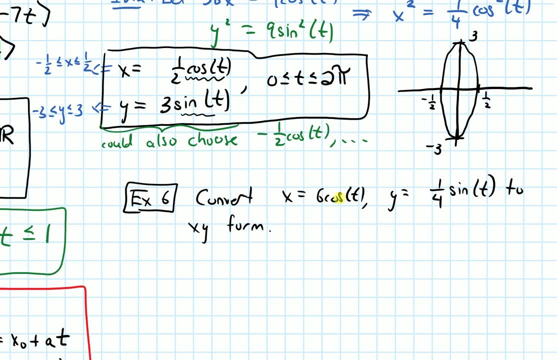 Alright, so let's do one more example in this video. So what if I was given something in parametric form- x equals 6 cosine t and y equals 1- fourth, sine t, and I needed to convert that to xy form. So this looks ellipse-esque, like I have something times cosine t and something times sine t. 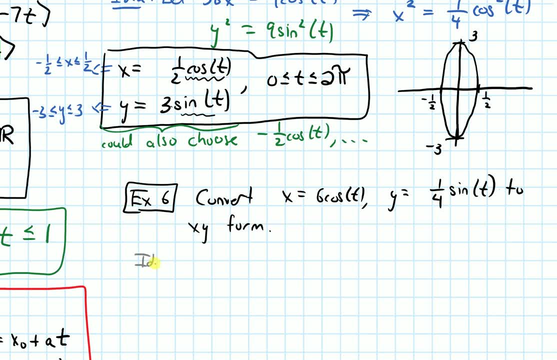 So we're thinking that it might be an ellipse. So here is the idea that we can use. The common theme to all of these has been that cosine squared t plus sine squared t equals 1.. If I want to convert this to xy form, I'm going to somehow have to get rid of this extra variable t. 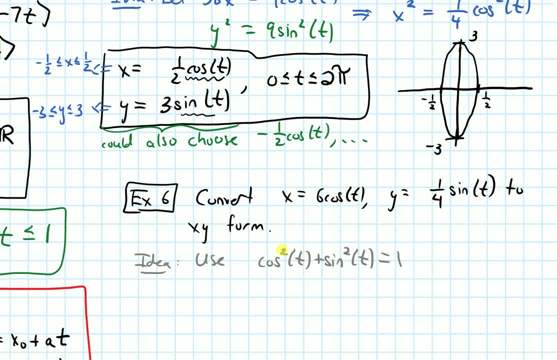 Alright. so one way I can do that is if I have an equation that connects the cosine and the sine, and this equation connects them, And I can figure out what cosine of t is on its own by dividing by 6.. So cosine of t is x over 6, and then cosine squared means we'll square that. 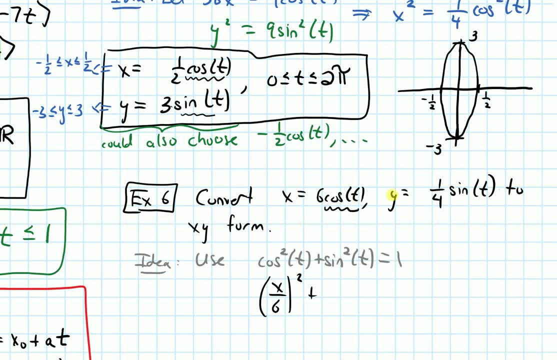 Similarly, sine of t, if you multiply over the 4, is 4 times y, And then we have to square that, because we have sine squared, And then this equals 1.. And now I can just simplify this a little bit. 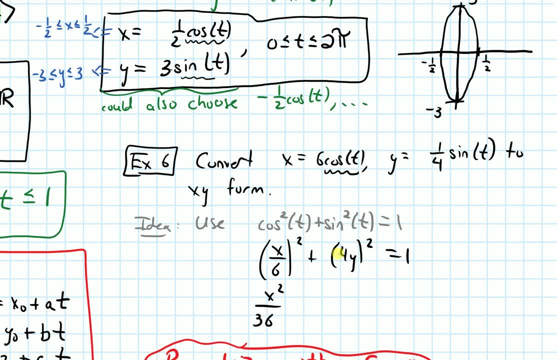 Simplify it a smidge and I get x squared over 36.. Squaring 4y, we get 16y squared equals 1.. And that is our equation, Purely in terms of x, Purely in terms of x and y.